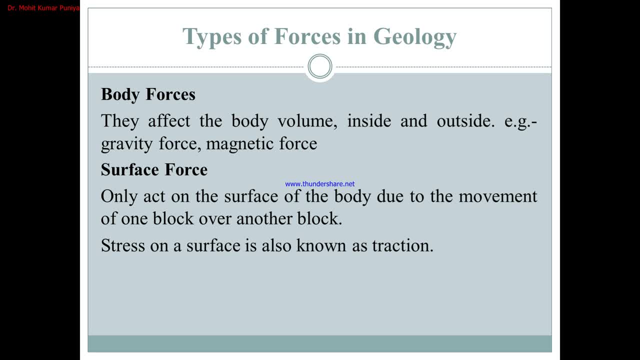 Body force are those forces, those affect the body from outside, inside, and change the volume also, For example, gravity force and magnetic force. Surface forces are those forces those act only on the surface, And these forces, these surface forces generated due to the movement of two blocks over one another. So such type of force is known as surface forces. 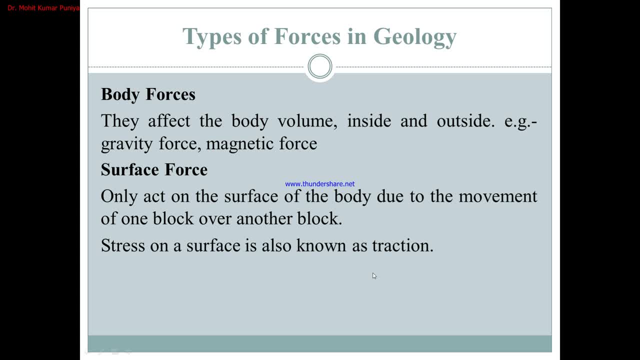 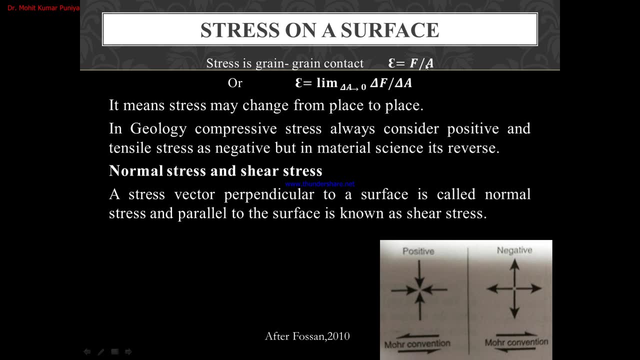 Stress on a surface is also known as traction, Then stress on a surface. Stress on a surface can be represented by F upon A Means force per unit area. But actually geology is homogenous, So stress is always changed from place to place. 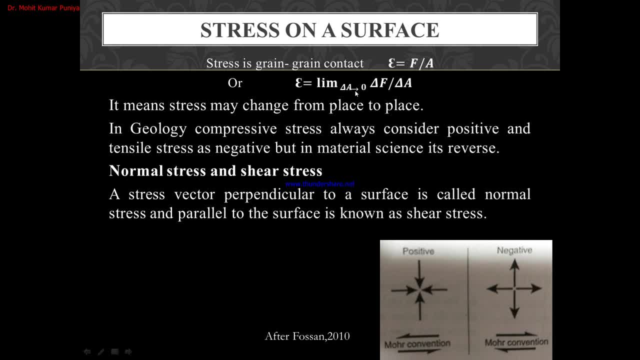 So we can represent the stress here: limit del A del 0, del F upon del A Del A. It means that stress change from place to place. In geology, compressive stress is always considered positive and tensile stress is negative, but in material science it is reverse. 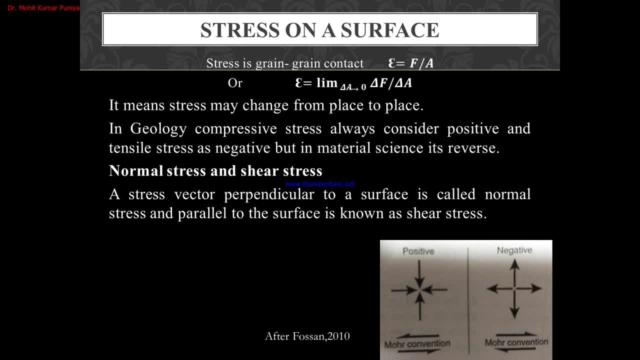 Compressive stress considered as negative and tensile stress considered as positive in material science, But in geology, compressive stress is always positive and tensile stress is always negative. A stress vector perpendicular to a surface is called a normal stress And parallel to the surface is known as the shear stress. 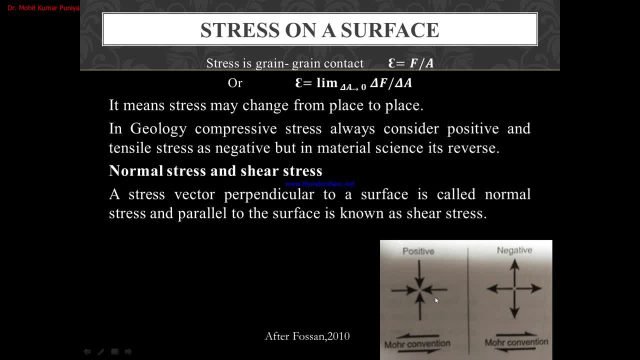 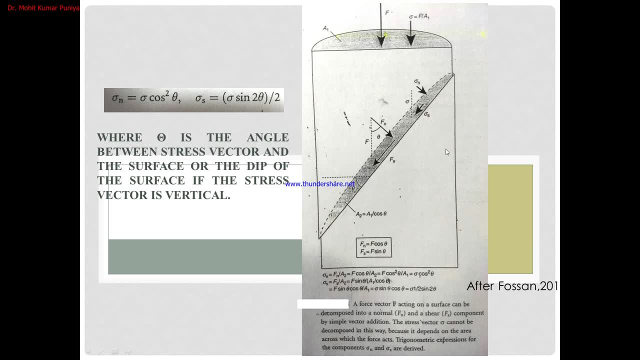 So this is the Mohr convention. We can see, this is the compressive stress, and this is positive, and these are the tensile stress, This is negative. So here we have one force acting on a surface. So, parallel to the surface, there are many vectors of the force. 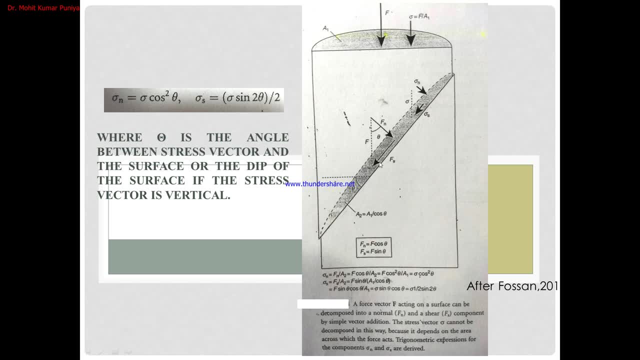 So that vector of the force, that acting parallel to the surface, that is known as shear force, And the vector that is acting perpendicular or normal to the surface, that is known as normal stress. Okay, Here the angle between the force and the normal is known as the theta. 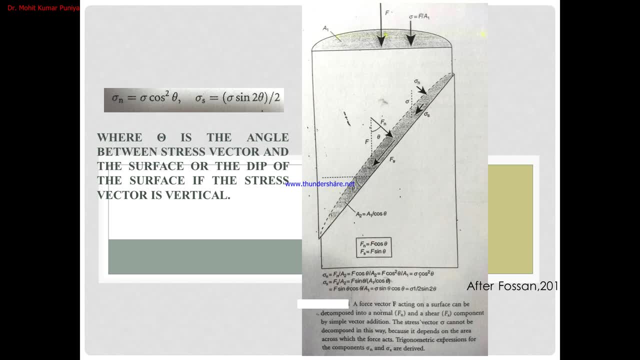 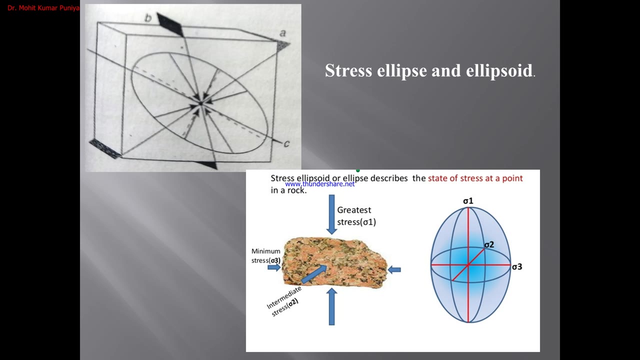 This theta angle is very important when we discuss about Mohr circular. Okay, So here normal stress can be represented stress cos, square theta and shear stress, sigma sine, 2 theta by 2.. Okay, Then there are infinite numbers of stress vector, and when we draw the mean vector of each plane on a point like this, an ellipse emerge in 2D. 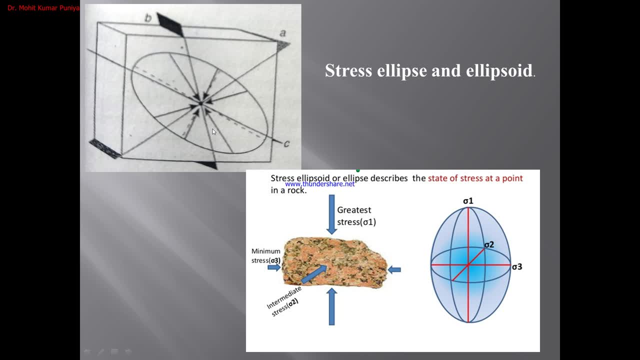 An ellipse emerge in 2 dimensions. The ellipse is called stress ellipse and the ellipsoid is called the stress ellipsoid. So in stress ellipsoid we can represent the sigma 1, sigma 2 and sigma 3.. Okay, So sigma 1, sigma 2 and sigma 3, axis also. 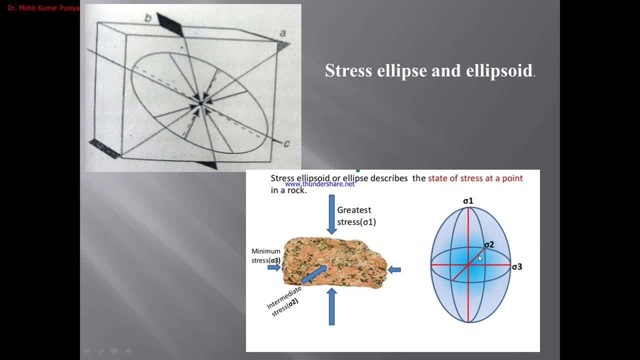 This sigma 1 is the principal stress axis, Sigma 2 intermediate, and sigma 3 is the minus stress axis. So here we can see, this is the foliated drop and this foliation represented here. This is the foliation direction. So this is the sigma 1 stress direction, greatest direction. 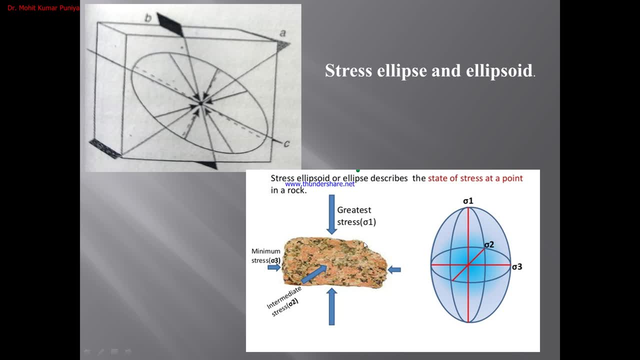 So the foliation orientation is like that. So why this foliation direction is like that? Because this is the strain axis, This is the stress axis. So strain axis and stress axis always perpendicular to each other. So here we are, applying the force from this direction. 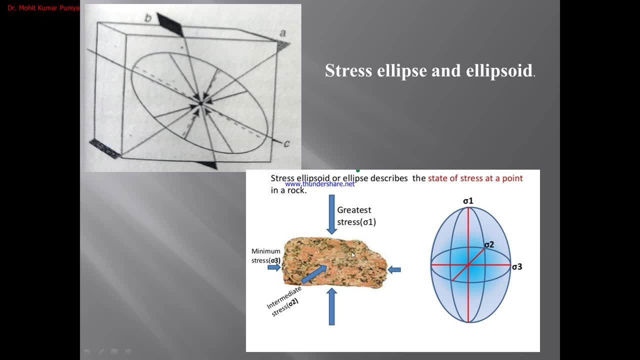 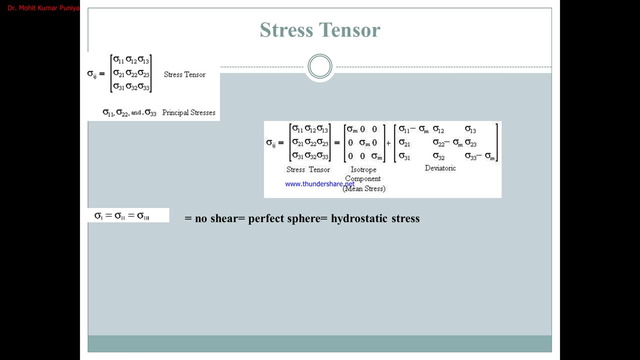 That's why we have more and more, or we can say most- deformation towards this direction. So this is the minimum stress direction, But when we talk about the strain, this is the principal strain direction. Okay, Now, This is the Stress tensor, or we can say this is the stress matrix. 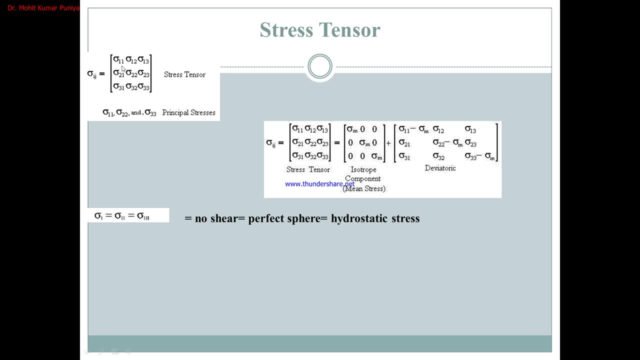 So we can represent the stress matrix at every point: Sigma 1, 1, sigma 1 2 by 3, by 3 matrix. So this whole matrix represent the stress tension. Here sigma 1, sigma 2 and sigma 3 are the principal stress axis. 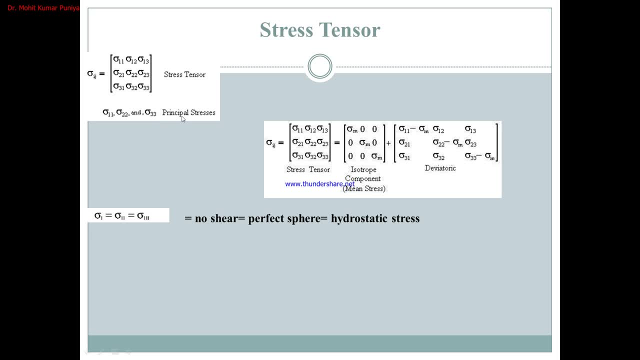 Intermediate stress axis and the minus minus stress axis. So here if we call this is the mean stress, If we take the mean stress, So mean stress we can represent by the matrix, like that: This is the stress tension. So the deodic stress is the deodic stress can be represented by stress tension minus mean stress, like that. 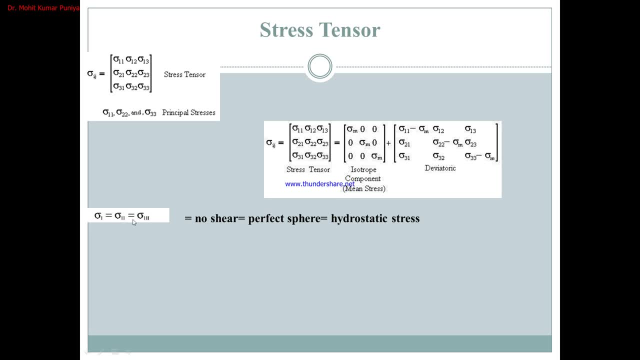 Okay, So if sigma 1 is equal to sigma 2 and sigma 3.. So that means that plane is perfect sphere. There is no shear, or we can say that is the hydrostatic stress Here. This is the Mohr circle. 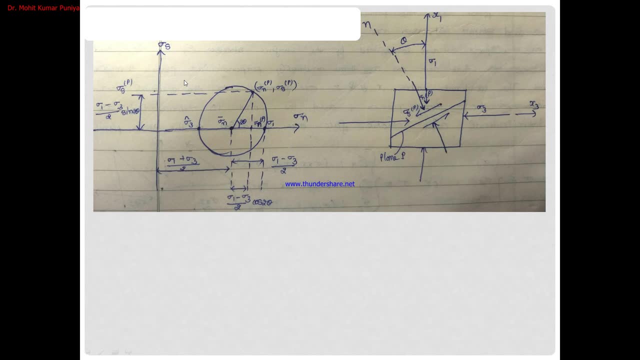 So, first of all, Mohr circle is invented by Moto Mohr, Otto Mohr. Otto Mohr was the German engineer, And by this German engineer This Mohr circle was invented in Mohr circle. Suppose that this is a plane. 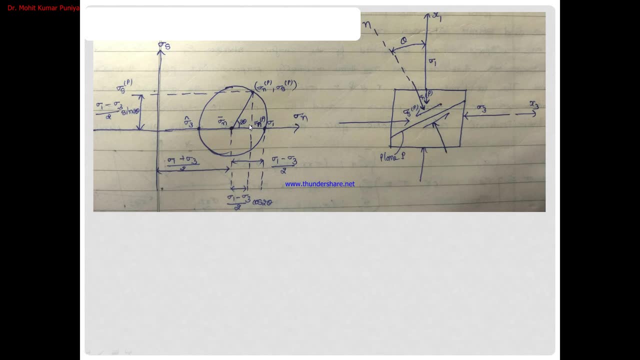 Here The incidence angle is the theta And here The incidence angle is the 2 theta. Here The diameter of the Mohr circle is principal stress direction: plus, minus, minus stress by 2. This is the mean of principal and minor. 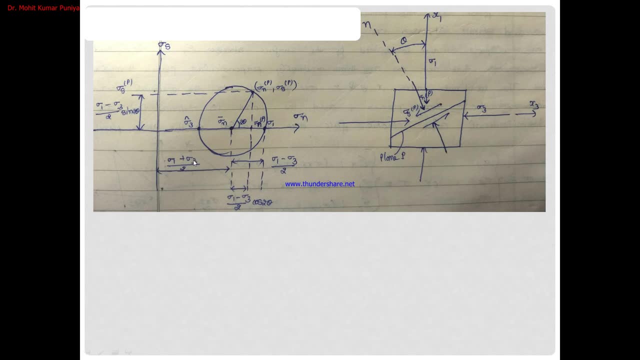 So if we take the diameter of the Mohr circle, That is principal stress and the minor stress. So we can. We have to plot the Mohr circle here, This 2 theta angle. Why this is 2 theta angle, We know by a theorem. 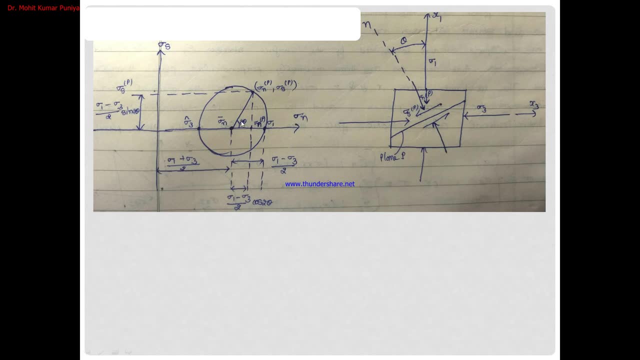 A theorem is say that The angle on a circle Will be the double To the angle of the periphery. Here- this is the point. We want to calculate the shear stress And the normal stress on this axis In the Mohr circle. 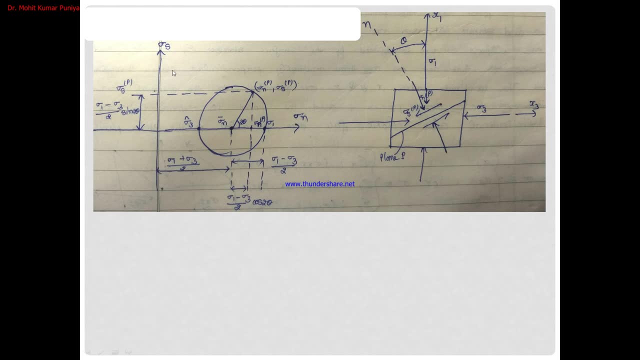 The horizontal axis represented by the normal stress, And the vertical axis represented by the shear stress. Let's take a diameter: sigma 1 plus sigma 3 by 2.. This is the diameter. So we have. We draw a circle here On this circle. 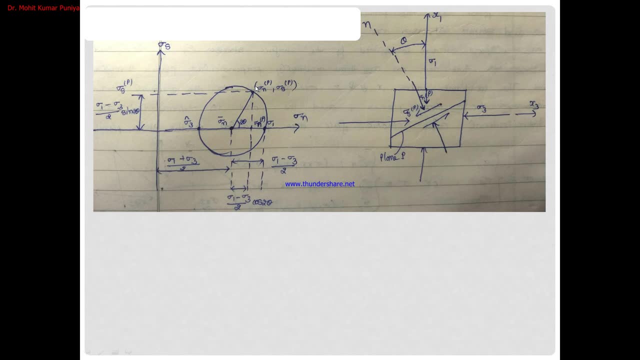 We have a point P. On this point P We calculate the normal stress As well as the shear stress. So here We apply a force. So the angle, The applying force And this point Make an angle, that is theta. 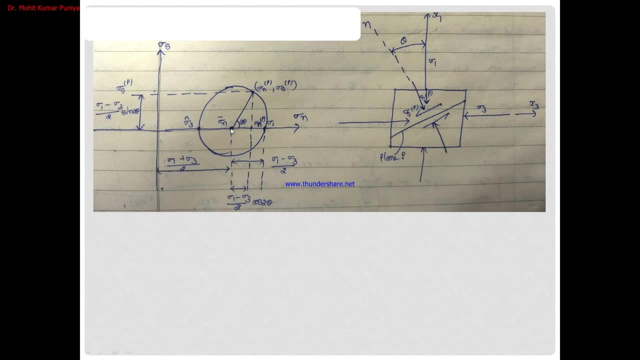 So this theta angle, If we reflect this on the center, It will be doubled. We know by the theorem The angle on the center Will be the double To the angle of the periphery. This is the 10th standard theorem. 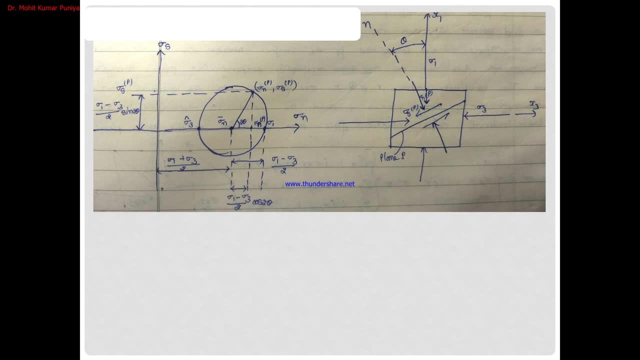 Okay. Or we can say: Kendra par bana cone, Pridhi par bane cone ka do guna hota hai. Okay, So, let's. So. the distance from the Shear axis To the center Will be sigma 1 plus sigma 3 by 2.. 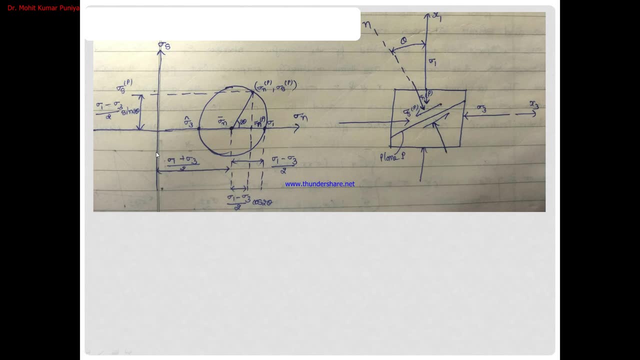 Because We have draw this Whole circle by the diameter. Okay, The distance from Principle stress to the center: Sigma 1 minus, Because this is the sigma 1.. And this is the sigma 2. And this is the sigma 3.. 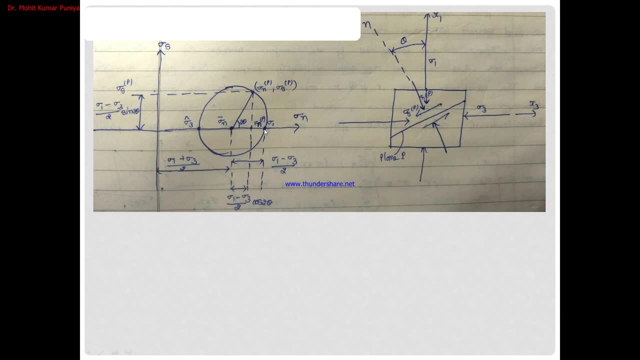 And this is the sigma 4.. And this is the sigma 5.. And this is the sigma 6.. And this is the sigma 7.. And this is the sigma 8.. And this is the sigma 7.. And this is the sigma 6.. 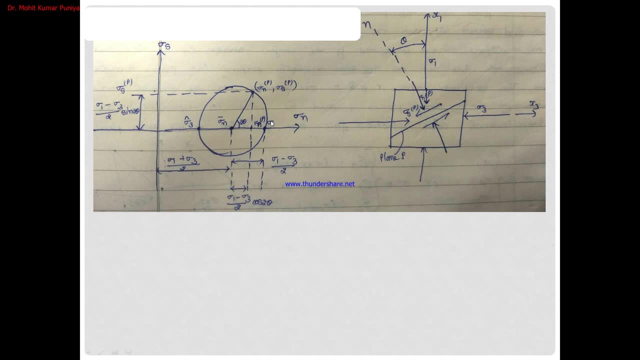 And this is the sigma 8.. And this is the sigma 9.. And this is the sigma 10.. And this is the Sigma 1 minus, Because this is the sigma one. So if you want to calculate, We have to take the mean from. 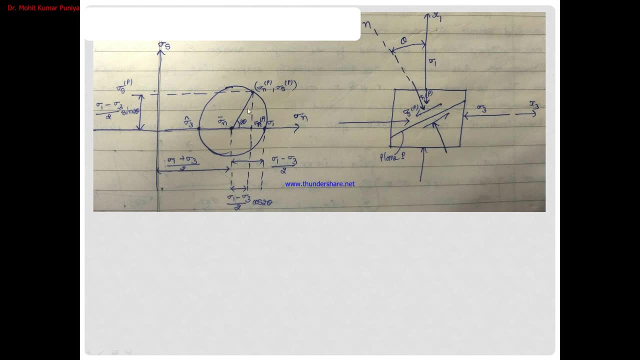 The principle to the minor one, So this will be sigma 1 minus Sigma 3 by 2.. If you want To calculate this distance From center point To the Normal of the This point, So here will be the normal. 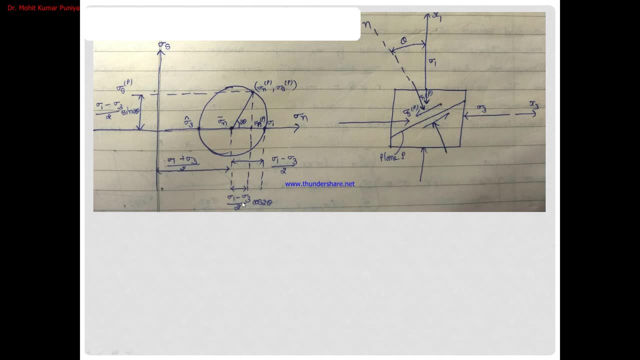 Stress For The point of P. So the Normal stress Will be sigma 1 minus Sigma 3 by 2.. Into cos 2, theta Similarly say the shear stress. So shear stress will be sigma 1 minus sigma 3 by 2, that will be sine 2. 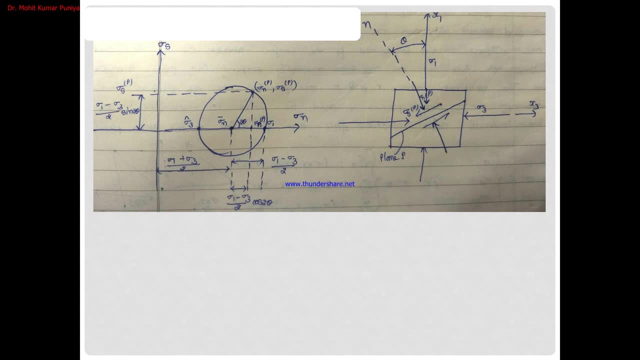 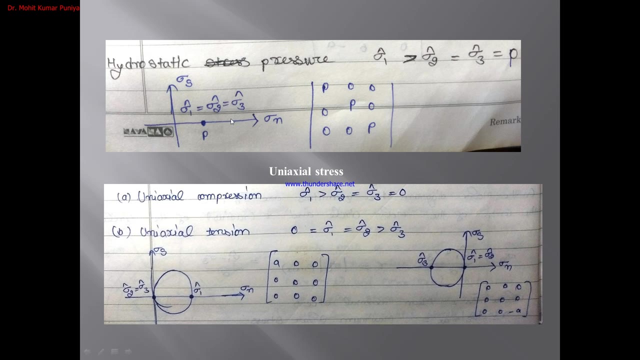 theta. So this is the simple nomenclature of the Mohr circle If we want to plot the different kinds of stress on Mohr circle. so what will be the representation? And this is the first case, for the hydrostatic pressure means there is: sigma 1 is greater than sigma 2 and sigma 2 and sigma 3. 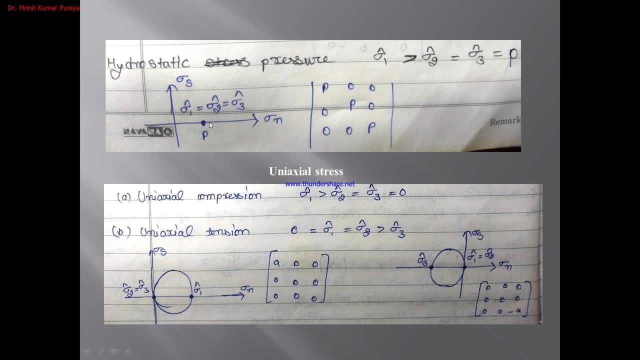 is 0. So here, this is the point: or sigma 1 or sigma 3 is equal to P, So this will be the point here. Actually, this is hydrostatic pressure. So hydrostatic press, there is shear stress component. 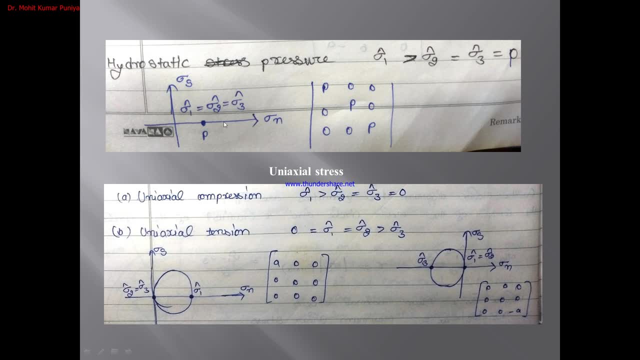 is 0. That's why it will represent on the normal stress axis direction and the matrix will be like this: Then: uniaxial compression: in uniaxial compression, sigma 1 is greater than sigma 2 and sigma 3, and sigma 3 is greater than sigma 2 and sigma 3 is greater than sigma 3.. So this is the. 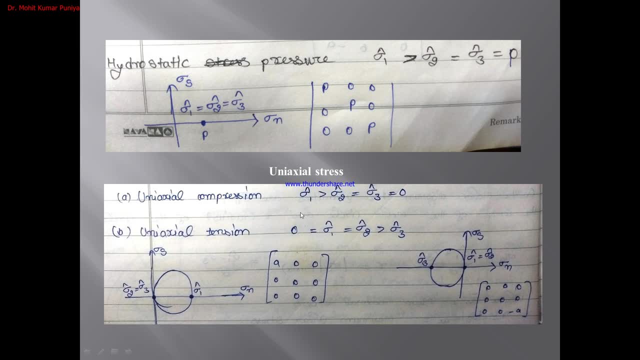 sigma 2 and sigma 3 will be 0. So in uniaxial direction, uniaxial compression, the nomenclature will be at the normal point and there will be no component of that means this circle will be represented here. This is the A condition for the uniaxial compression. Sigma 2 and sigma 3 is the 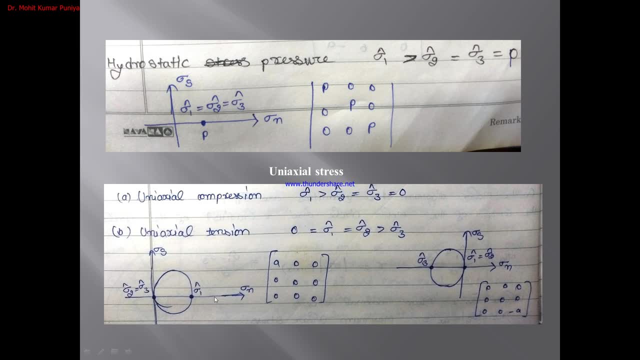 0.. Sigma 1 is greater than sigma 2 and sigma 3 and not equal to 0.. So this is the uniaxial compression condition, and here uniaxial compression can be represented by the matrix means. uniaxial compression means only one component is a unit, other, all the components will be 0. 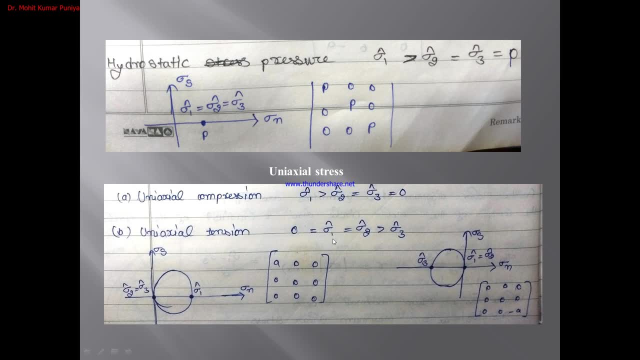 Then uniaxial tension: in uniaxial tension, sigma 1, sigma 2 will be 0 and sigma 3 will be greater than, or I mean will be less than to the 0. So this is the representation here. we can see. this is this. 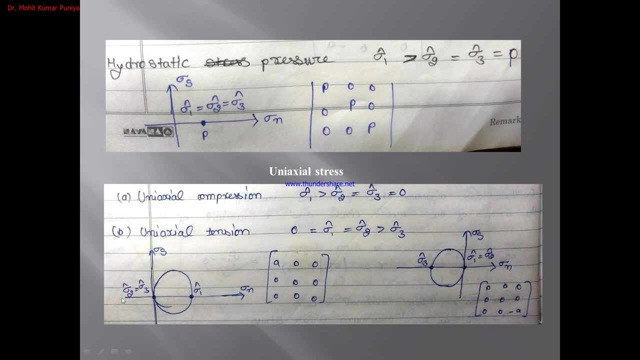 horizontal axis. So if we move towards the left direction it will be minus. and if we move on the shear stress axis towards the downside from the center point it will be minus. So tension always create in the negative points. So here this is the negative axis, So the Mohr circle will be flowed towards. 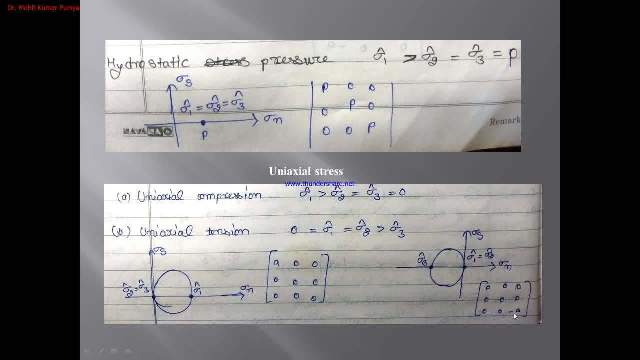 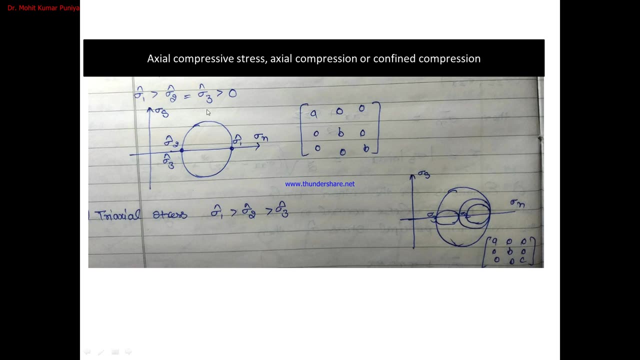 the negative direction and by the matrix it will be represented by negative mass here. Okay, then axial compression, stress. So axial compression or confined compression. In this case sigma 1 will be greater than sigma 2 and it equal to sigma 3, but sigma 3, this is non-zero condition. So in the on the Mohr circle, 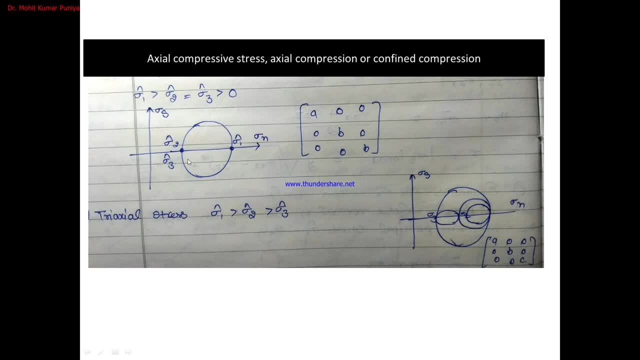 we can represent such type of condition like this. This is a Mohr circle. Here sigma 1 is the greater than to the sigma 2 and greater than sigma 3, and sigma 2 and sigma 3 is non-zero condition. So this is the axial compressive stress, or axial confined compression. 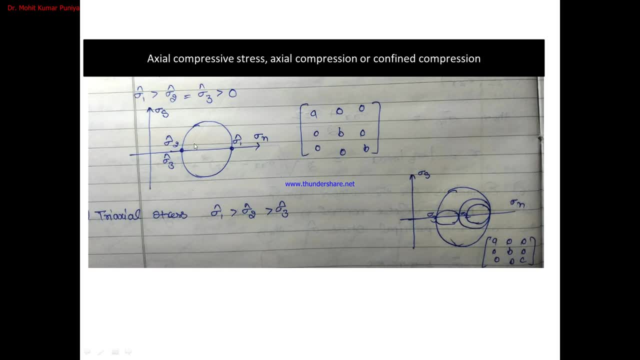 So by the matrix A, B and B, because sigma 2 and sigma 3 is equal. that's why we have given the same number here. Then triaxial stress means sigma 1 greater than sigma 2 greater than sigma 3.. 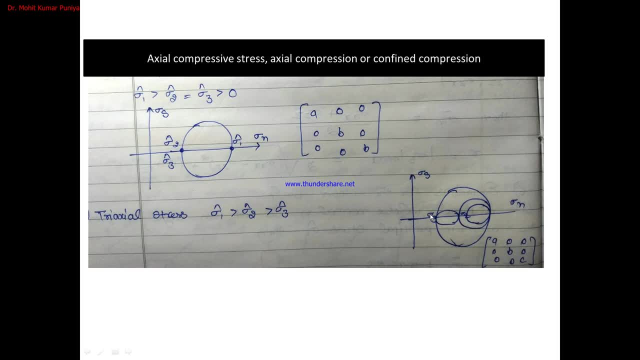 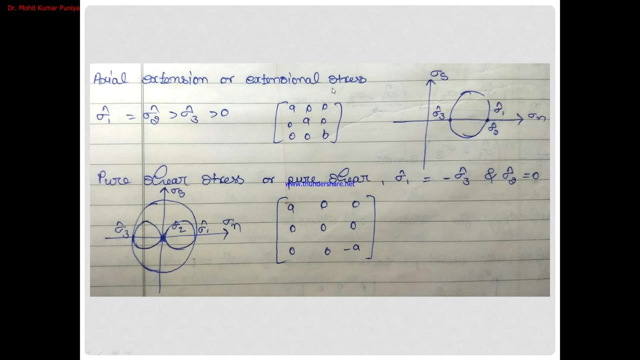 Here this is sigma 1, then we have sigma 2, then we have sigma 3.. So for the stress matrix we have given all the numbers in different different A, B and C, Then axial extension: in stress, axial extension or extensional stress, sigma 1 is equal to sigma 2 and sigma 2 greater. 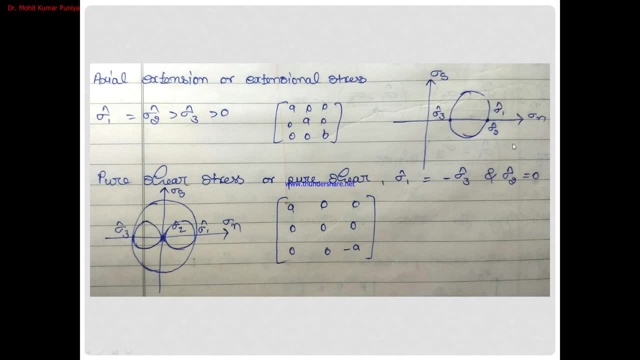 than sigma 3 in the matrix A, A and B. So sigma 1 and sigma 2 will be at the same point and sigma 3 is non-zero. that's why it will be here. So we can represent by the Mohr circle like that. 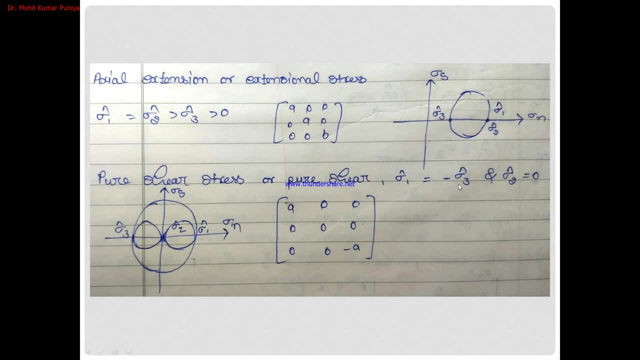 Then pure shear stress, or pure shear. sigma 1 is equal to minus, sigma 3 and sigma 2 is equal to zero. So here we can represent the two circle that one is towards the positive axis, another one is towards the negative axis, and the common point. 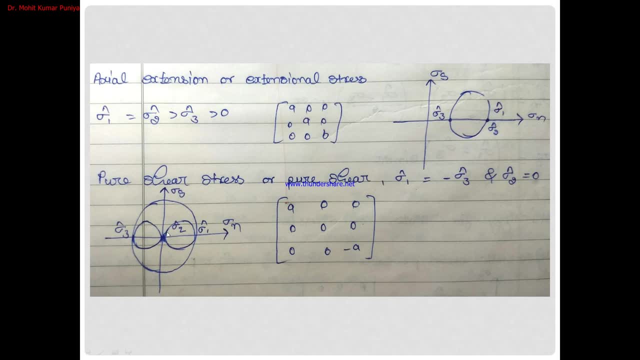 will be passed through the zero point. So this is here. sigma 2 is zero for this circle and for this circle also. Here, sigma 1 is the greater than sigma 3, equivalent to sigma 3.. The value of sigma 3 on both the axis, towards negative and positive, will be the same for the pure shear. 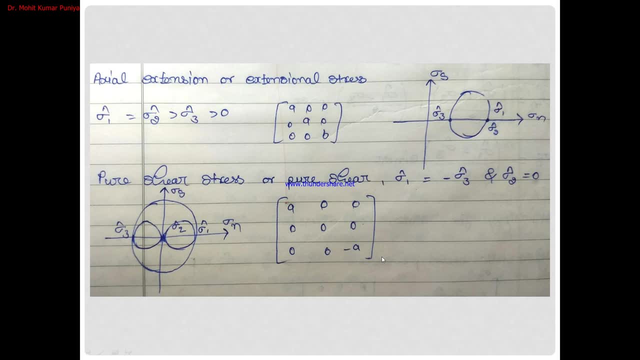 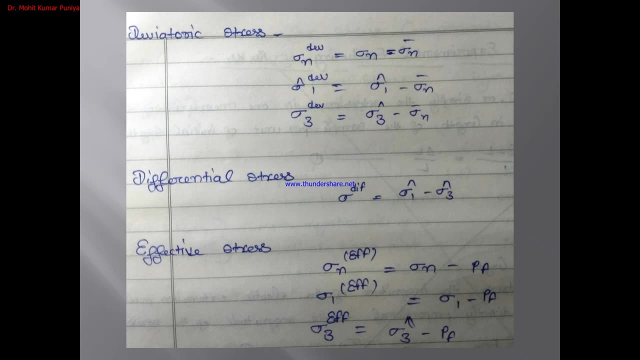 stress And for the matrix A and minus And P will be zero, because this is sigma 2, sigma 2 will be zero here. Then deviatoric stress. Deviatoric stress can be represented by sigma n, where sigma n is equal to. 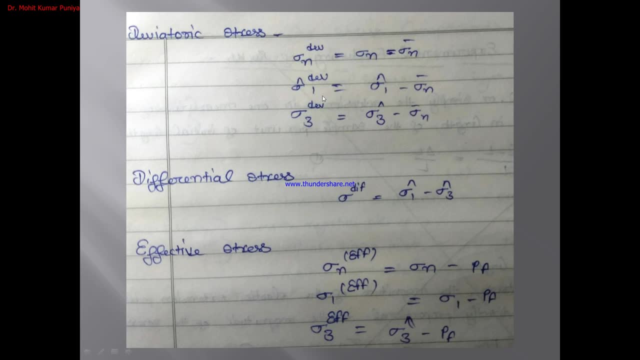 sigma n is equal to. so we can represent that sigma 1 is equal to sigma 1 minus sigma n. This is the mean stress, So we can represent the deviatoric stress from the stress tension minus mean stress. Then differential stress, So we can represent the differentiated stress from the stress tension. 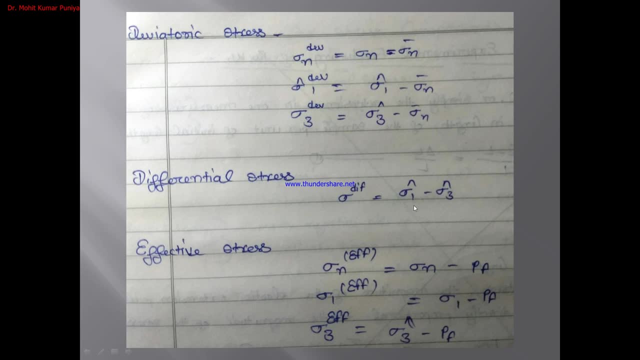 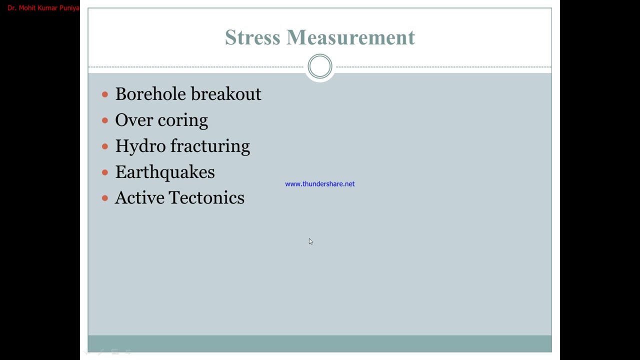 stress. differential stress will be sigma 1 minus sigma 3, because sigma is the principal one and this is the minor one. so differential stress can be represented like that. then effective stress. effective stress will be: sigma 3 is equal to sigma 3 minus pf. okay, then stress measurement. 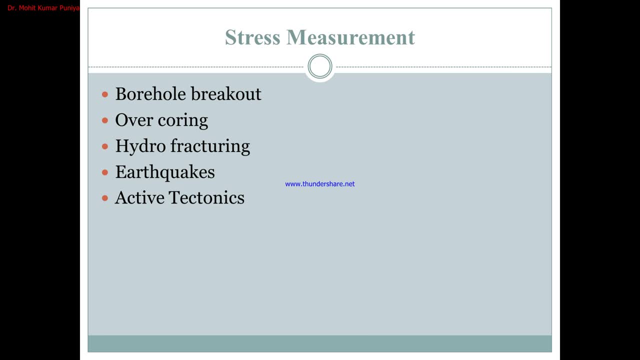 now, these days we can measure the stress and this stress measurement is very important for the civil structure. suppose that we are going to construction. we are going to construct the civil structure in the high stress stress region. those are tectonically active. okay, so tectonically active region if we meet our structure along the principal stress direction, the stress. 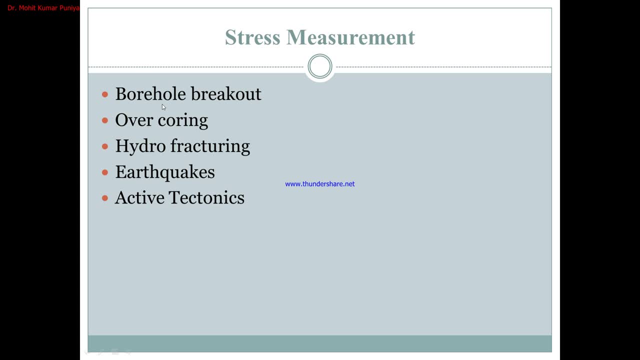 will create the more and more damage to towards our structure. so the stress measurement is very, very important for the mega civil structure, if those structures laying in the high structure active regions okay, or so here are some methods so based on these methods we can measure the principal stress or stress directions. borehole breakouts: borehole breakouts is very common. 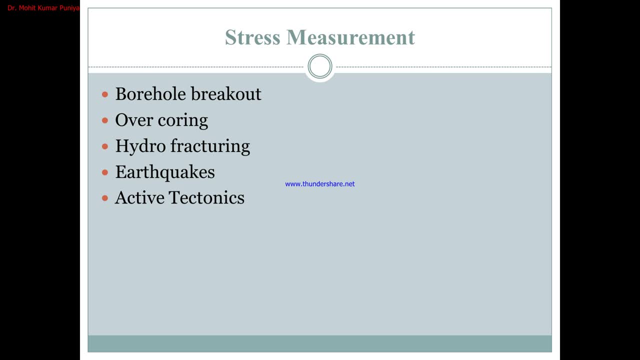 phenomena for the hydrocarbon, hydrocarbon exploration. so because in hydrocarbon exploration we drill up to three to four kilometers. so below three to four kilometers there is too many active stresses. so based on the sensors and based on the distortion of the borehole, we can measure how much stress is acting on the boreholes. 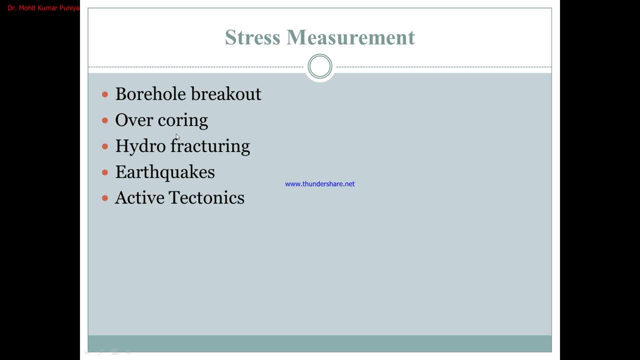 then overcoring. here, in overcoring method we drill one core at larger size that will be- means a standard is 76 mm. then we drill another borehole within that borehole that will be smaller than the outer one. that is 36 centimeter mm. so upper portion is made by 76 mm and the lower portion 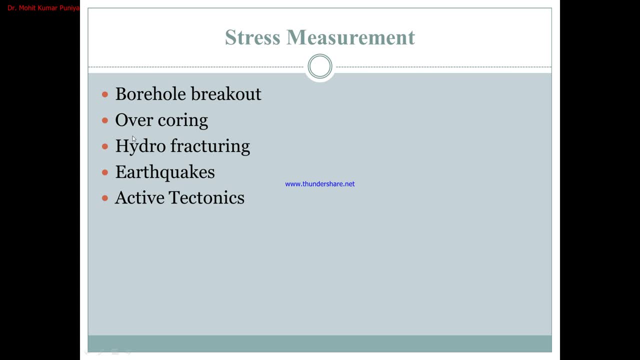 has dimension 36 mm. so we plot, we install those sensors there and sensor detects the distortion in both the boreholes and we compare the distortions and we calculate where it is present in each direction in the boreholes. have not holding hydro fulfilled hydro flexuring. see, actually hydro flexuring is the phenomena where weЙ artificially, We try to feel the rocks. 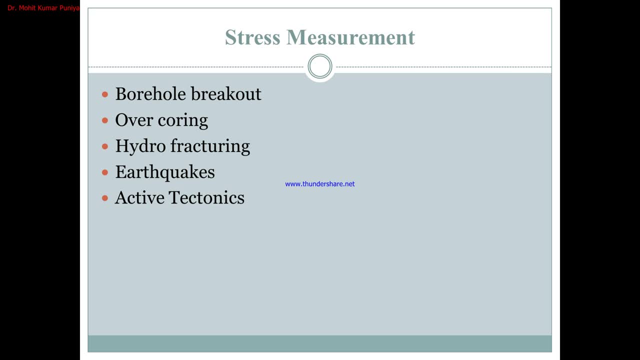 We artificially try to feel the rocks. we try to feel the rocks so very, try to fill them, and that also can be due to realizing that we can damage the softlyßh kidd ones that we cannot fabricate at all levels of the rock pores或者 fö pasteur αν ans inhale něn Rochester. we can also save those to flood the local rock supermarket we will place at design and present it. we can try to take the unique eats on one part or another part of this bed using the